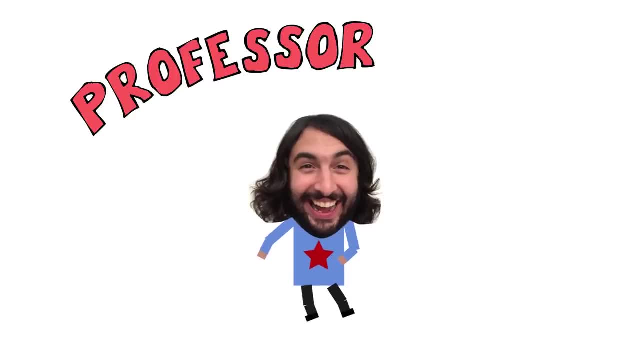 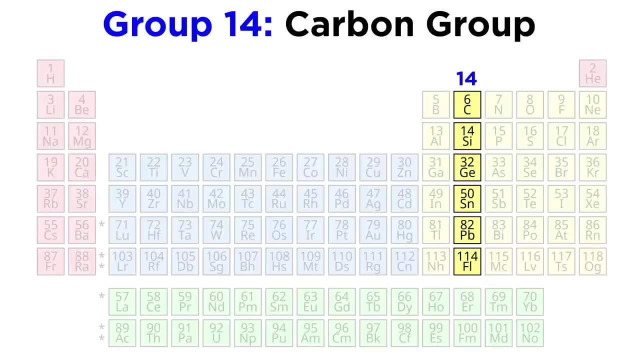 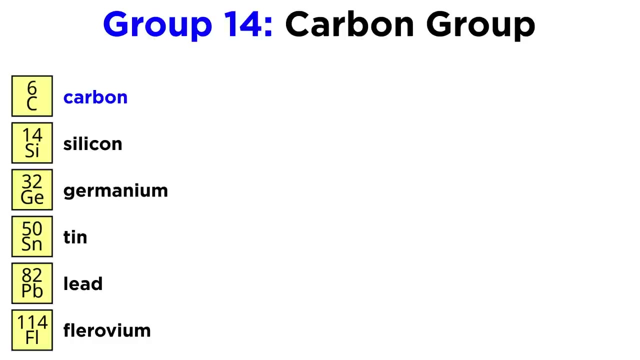 With Groups 1,, 2, and 13 covered, it's time to visit Group 14.. This is known as the carbon group, since carbon sits right at the top. The other members of this group are silicon, germanium, tin, lead and fluorovium. These elements have electron configurations that end in. 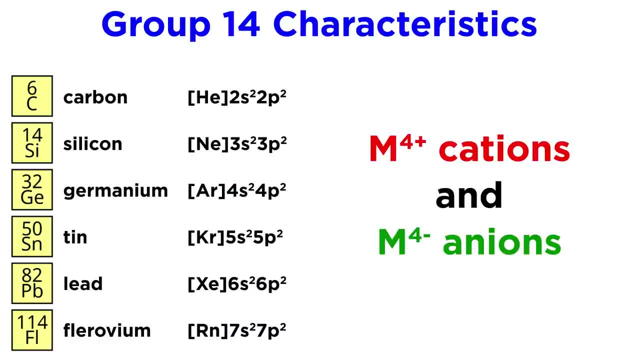 ns2 and p2, and they are quite interesting in that both 4 plus and 4 minus ions are possible, depending on what they are interacting with In terms of oxidation states. plus four is all that carbon and silicon will exhibit, while germanium, tin and lead can exhibit both plus four and plus. 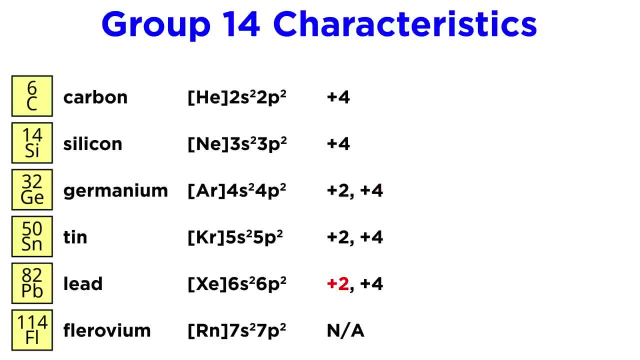 two, with plus four being more common, except for in lead, where plus two becomes more common due to the inert pair effect. Again, this is where the S electrons in the outermost shell tend to remain unshared in post-transition metals. In this group we also encounter our first non-metal apart from hydrogen. 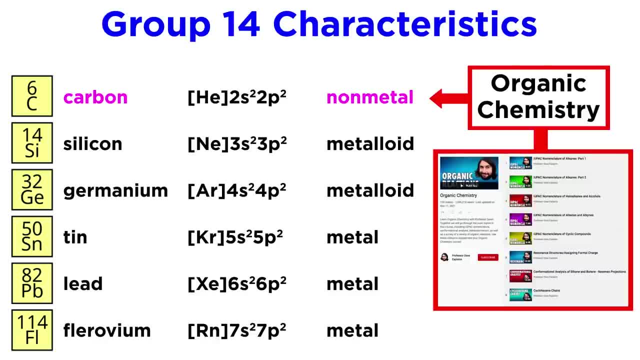 and that is the ubiquitous carbon which we know so much about from organic chemistry. Since that entire series was essentially all about what carbon can do, we won't bother summarizing any of that here. Silicon and germanium, on the other hand, are both metalloids. 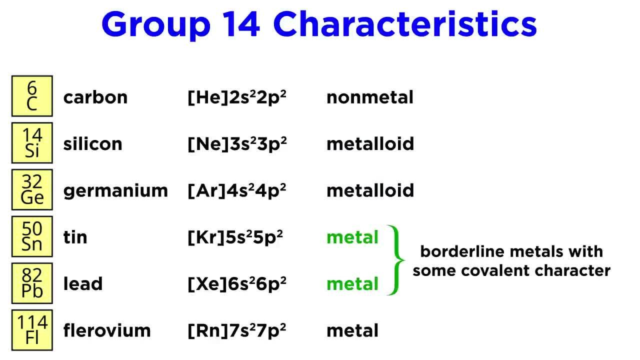 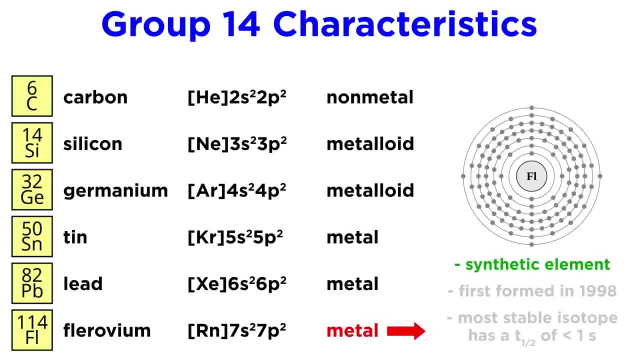 that often form covalent bonds, while tin and lead are borderline metals that have significant covalent character. Fluorovium, like nihonium from the previous tutorial, is a synthetic transactinide element that was first formed in 1998.. It is extremely radioactive. 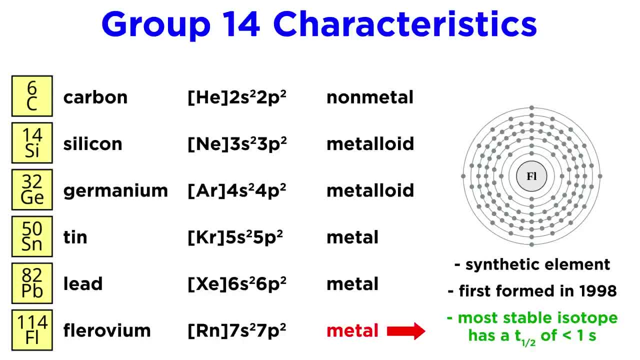 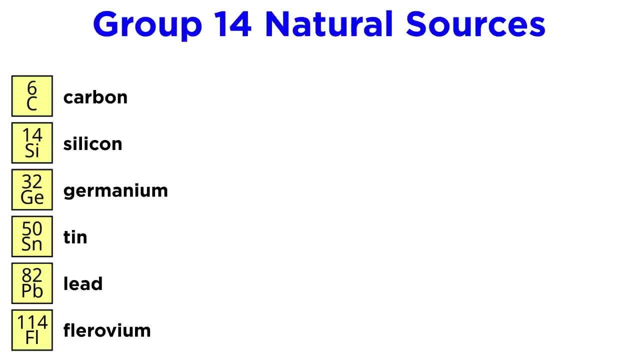 with the most stable isotope having a half-life of just under one second. so there is essentially nothing to discuss in terms of reactivity and applications. So where can these elements be found? As we mentioned, carbon is just about everywhere, especially in living. 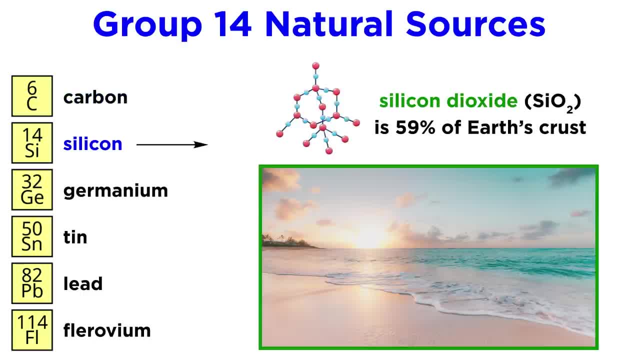 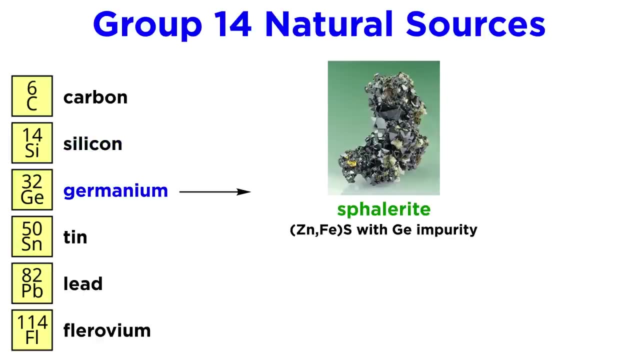 organisms which are carbon-based. Silicon is even more abundant in the form of silicon dioxide. This actually makes up 59% of Earth's crust and is easily found in sand at any beach. Germanium is found in ores like sphalerite, which has germanium sulfide impurity. 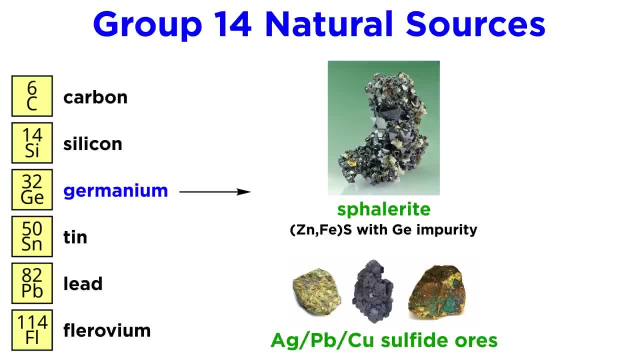 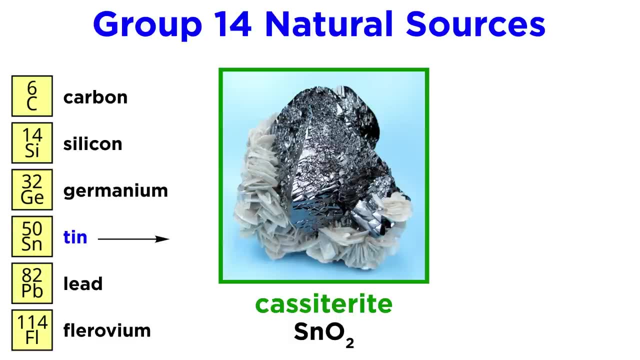 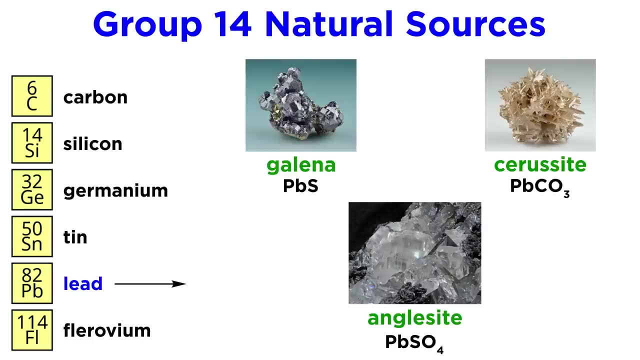 as well as silver, lead and copper sulfide ores. Russia and China are primary producers. Tin is available in the form of cassidorite, found primarily in China and Indonesia, And lead is found in ores like galena, cirrosite and anglicite. 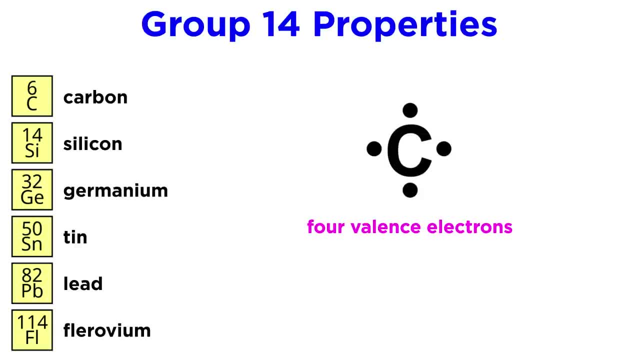 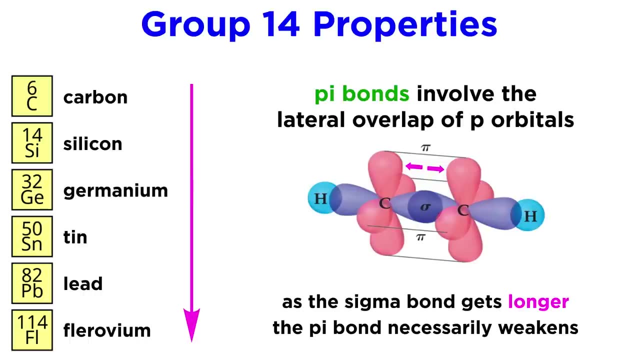 To get into bonding behavior. the elements in this group all have four valence electrons, which allows for a range of hybridizations and therefore diverse structures. For example, pi bonds are possible between adjacent p orbitals. As we go down the group, these outermost p orbitals become larger, but they also get further away from one another. 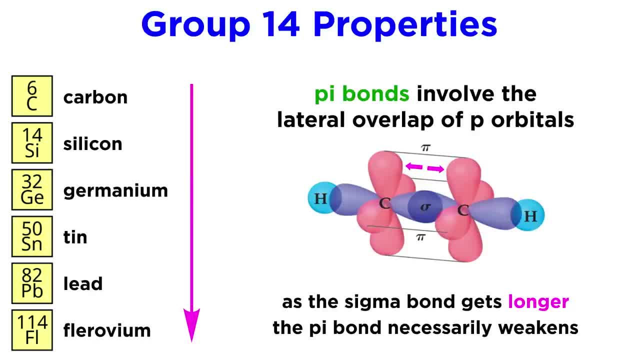 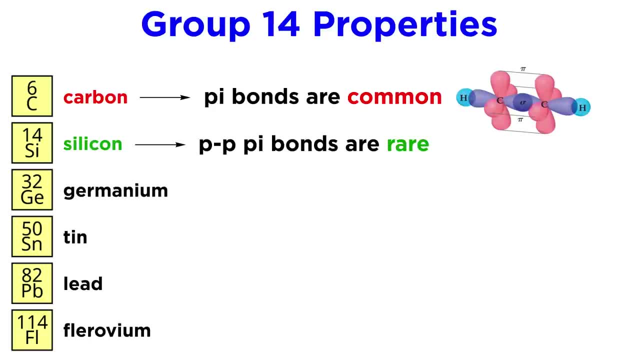 as the covalent bond length increases. This weakens the interaction. thus, while pi bonds are very common between carbon atoms, they are already quite rare between silicon atoms. On the other hand, pi bonding between one p orbital and one d orbital is also possible. 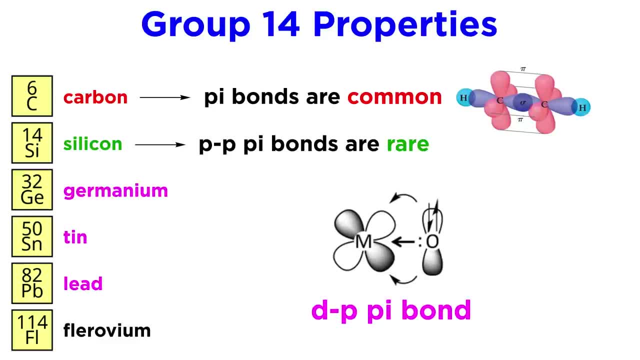 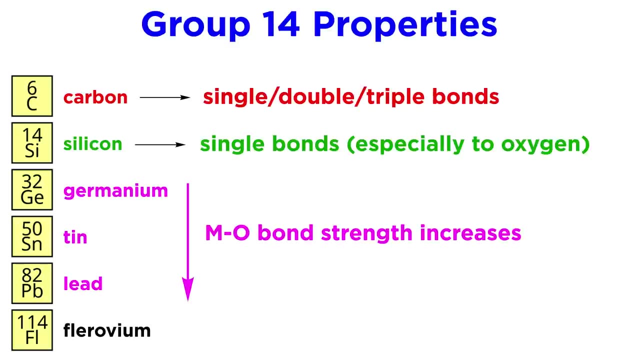 and this actually strengthens going down the group as these orbitals get bigger due to the angle in which the lobes of the d orbitals project and the resulting enhanced overlap with the p orbital. So while carbon readily forms double and triple bonds, silicon prefers single bonds especially. 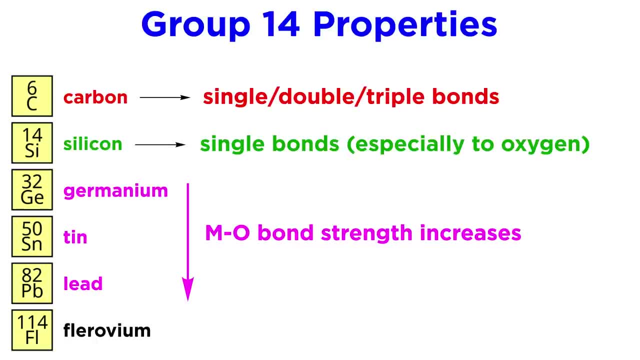 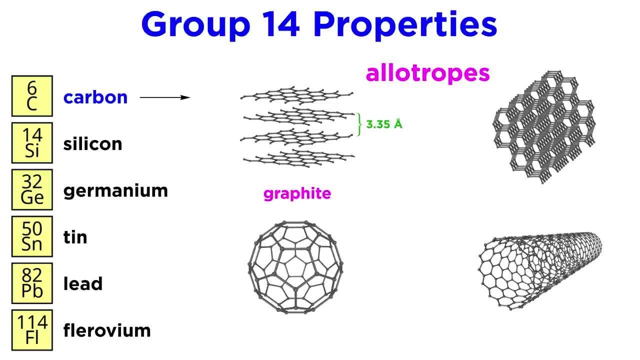 with oxygen and metal-oxygen bond strength increases going down the group. Continuing with elemental forms, carbon has several common allotropes. First there is graphite, which consists of sheets of fused benzene rings around three point two. These layers make electrostatic interactions but slide very easily over one another, giving 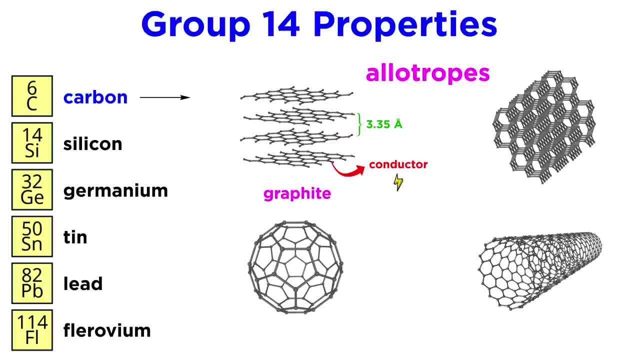 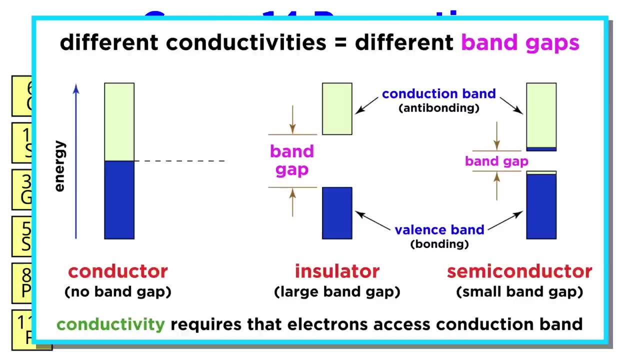 graphite application as a lubricant. This extended pi system makes graphite a semimetal with some overlap between its valence band and conduction band, so it is also able to conduct electricity. Visit my general chemistry tutorial on conductors, insulators and semiconductors if you wish. 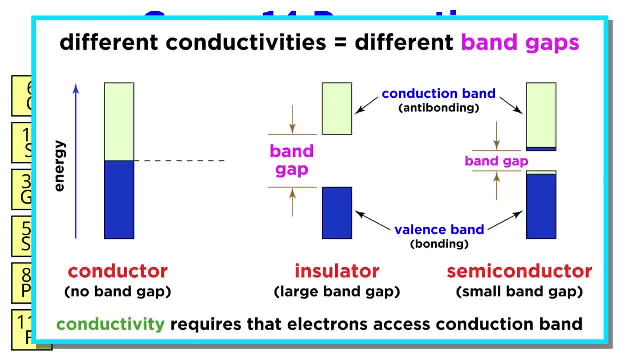 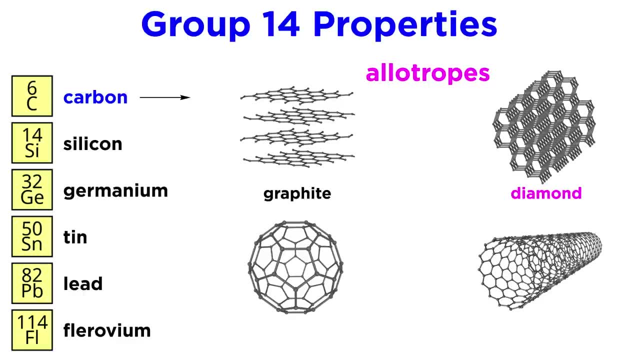 to review information regarding molecular orbits. Diamond is an extended lattice of sp3 hybridized carbon atoms, making this one of the hardest and most durable substances known. Then, a bit more exotic are the fullerenes, such as Buckminster fullerene, commonly referred. 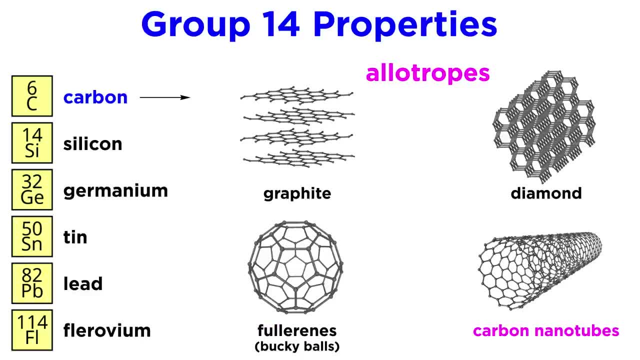 to as buckyballs, as well as things like carbon nanotubes, which have astonishing tensile strength. These have tremendous application in nanotechnology and are the subject of ongoing research and research in the field of nanotechnology. In addition, they are also known as buckyballs or buckyballs, or buckyballs as well as things. 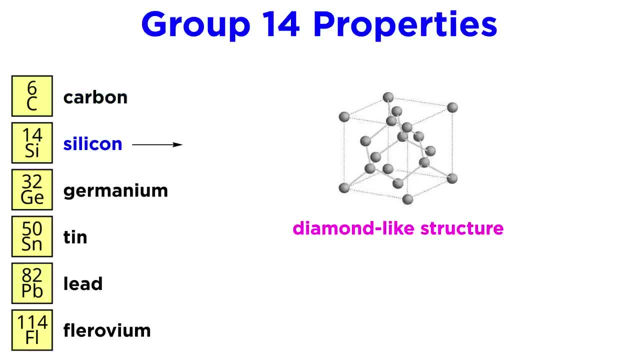 like carbon nanotubes, which have astonishing tensile strength. They are also known as buckyballs or buckyballs or buckyballs. as well as things like carbon nanotubes, which have astonishing tensile strength, Silicon also takes on a diamond-like structure and is a semiconductor due to the small. 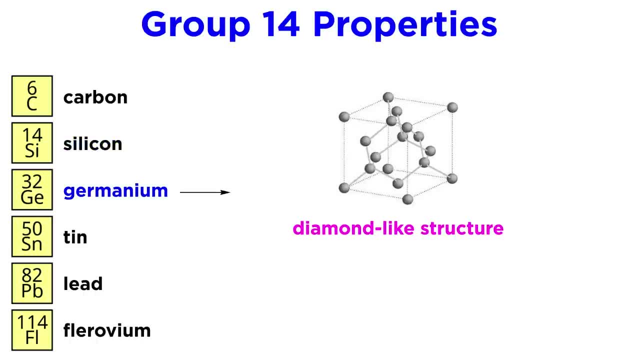 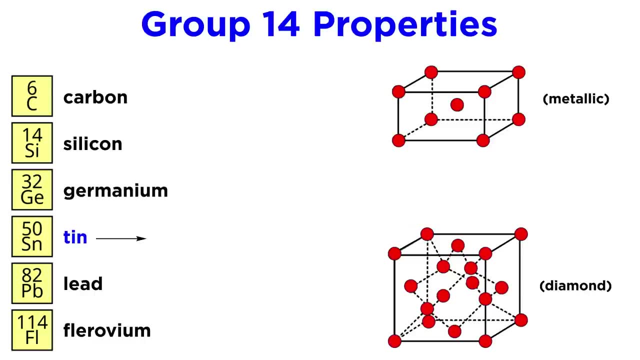 band gap between its valence band and conduction band. Germanium also has a diamond-like structure, while tin has both metallic and diamond allotropes which are stable. The metallic is malleable and shiny, while the diamond is brittle and gray. 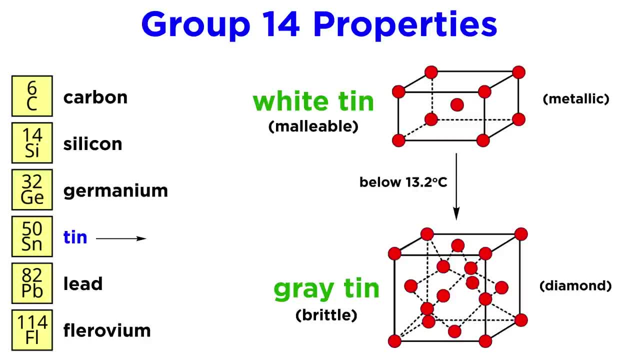 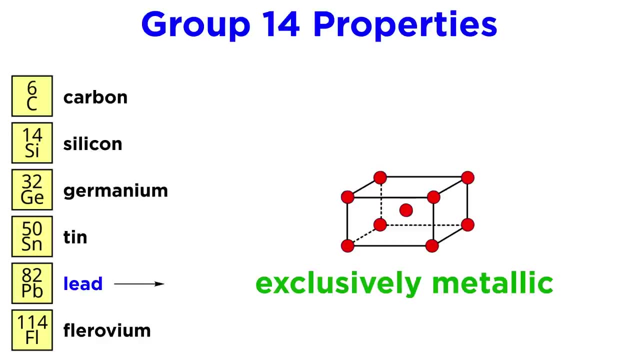 Cold weather encourages transition from the metal allotrope to the diamond, which is why objects made of tin tend to disintegrate in cold weather and in catalytic fashion, a phenomenon known as tin disease or tin pest. Lead, unlike tin, is exclusively metallic and less reactive than the other metals in 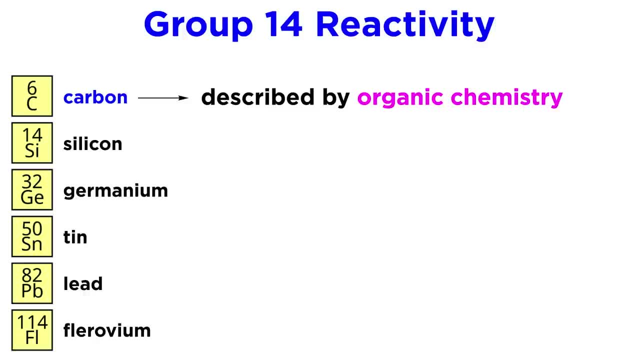 this group. Now, in terms of reactivity, again, we don't need to say much about carbon, since that's what organic chemistry is for, but we want to be aware that, beyond its covalent bonding behavior, carbon atoms can interact with each other. 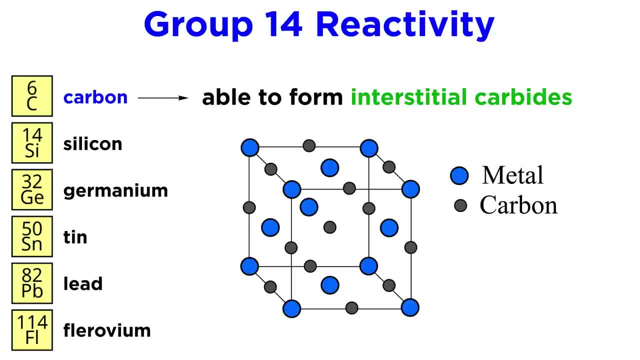 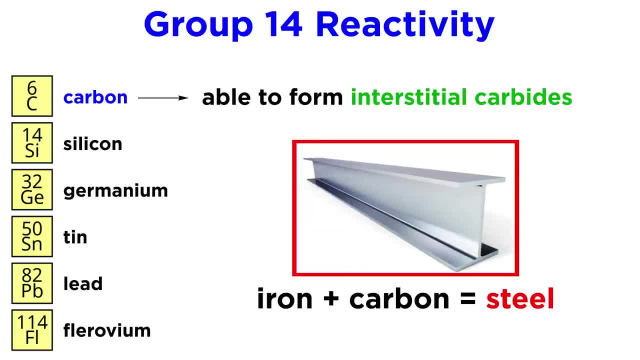 Carbon atoms can interact with transition metals to form interstitial carbides, where carbon atoms fit into octahedral holes in close-packed metal lattices. This produces alloys that are very hard and with high melting points, such as when combined with iron to make steel. 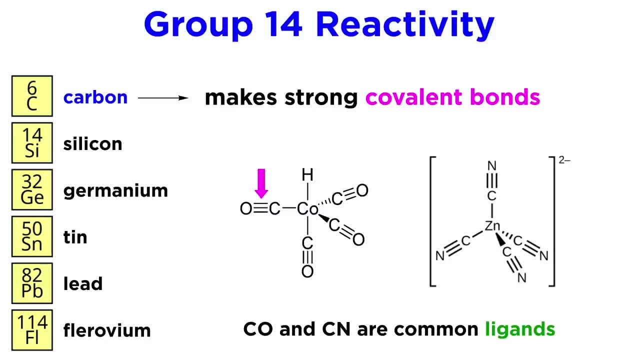 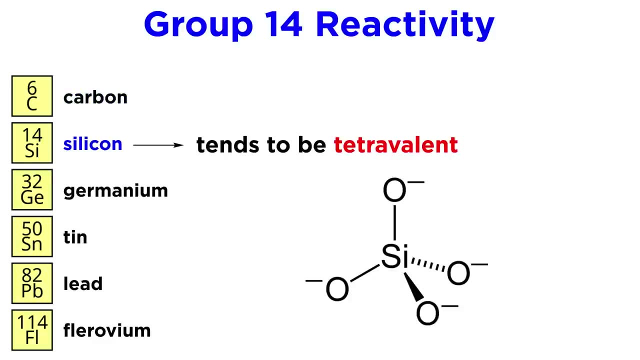 Covalently speaking. carbon-oxygen bonds are extremely strong and we will see the CO ligand in many transition metal complexes. Carbon-nitrogen bonds are also strong, so we can say the same for silicon. Thanks for watching. Silicon is similar to carbon and therefore tends to be tetravalent, but with an extra. 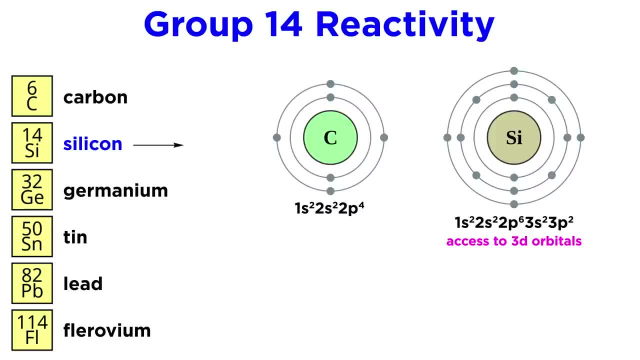 shell. it has occupied d orbitals, which makes for easy hybridization and changing of geometry. More atoms can fit around the larger silicon atom than the smaller carbon atom. This means silicon can be pentavalent, while carbon cannot save for fleeting moments under. 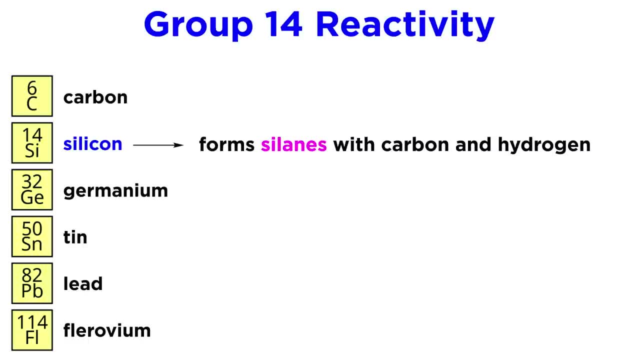 certain extreme conditions we will not discuss here. Silicon will bond with carbon and hydrogen to form silanes such as tetramethylsilane or TMS, which should be familiar from our study of NMR spectroscopy. Like carbon, silicon makes very strong bonds to oxygen, so these are quite common. 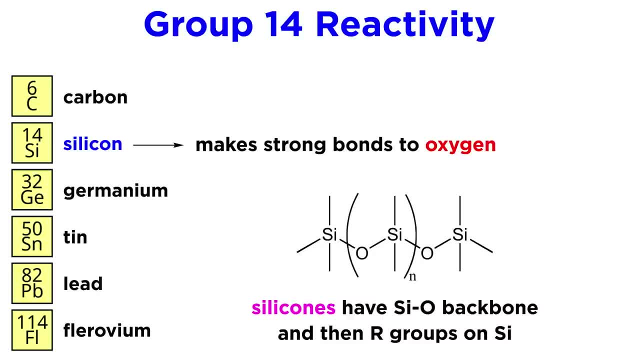 Silicones are compounds with a silicon-oxygen backbone and are groups attached to the silicon atoms, And silicates are salts in which the anion contains silicon and oxygen. These compounds are called silicon bonds. These are abundant in Earth's crust and are studied in detail over in the geology. 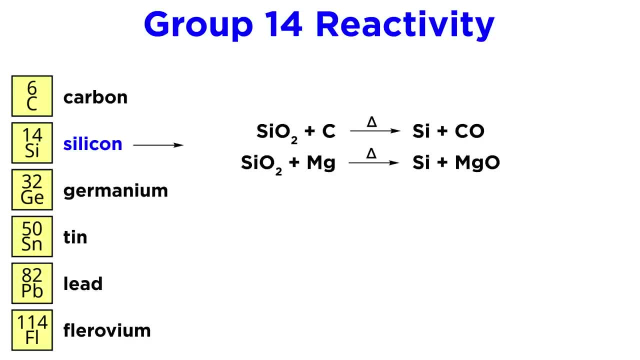 series. It is possible to produce pure silicon by the high temperature reduction of silicon dioxide with a strong reducing agent like carbon or magnesium solid, which yields silicon and either carbon monoxide gas or magnesium oxide solid. In terms of applications, again for carbon, these are limitless, given carbon's omnipresence. 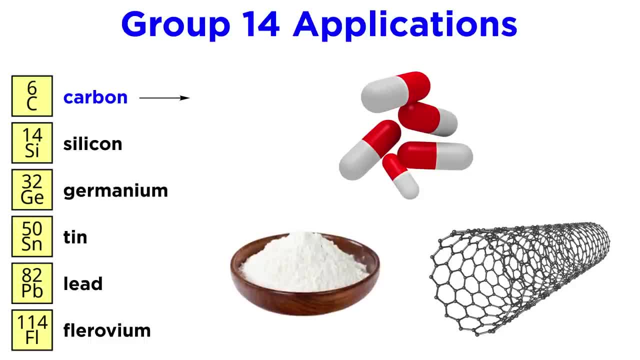 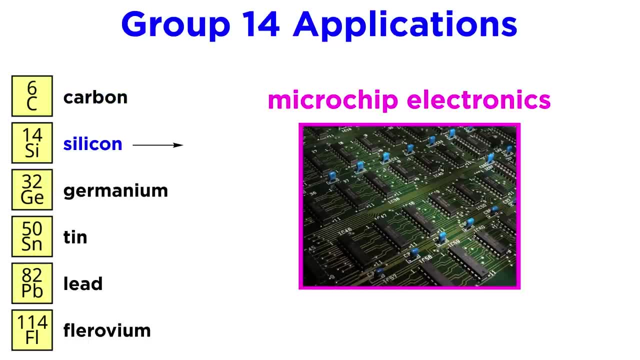 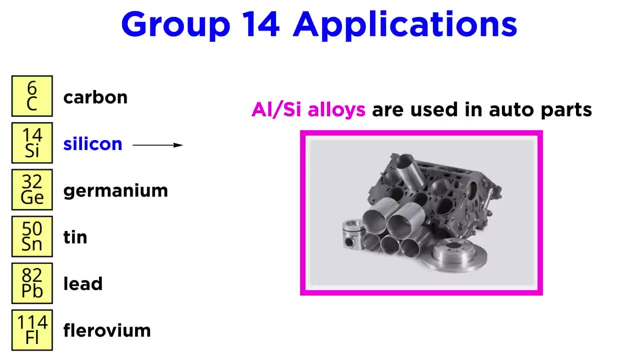 in natural products, drugs and the exotic allotropes we mentioned. For silicon. the applications should also be quite familiar, as it is crucial for microchip electronics and therefore virtually every bit of advanced technology we use every day. Silicon is also used in aluminum-silicon alloys for auto parts. 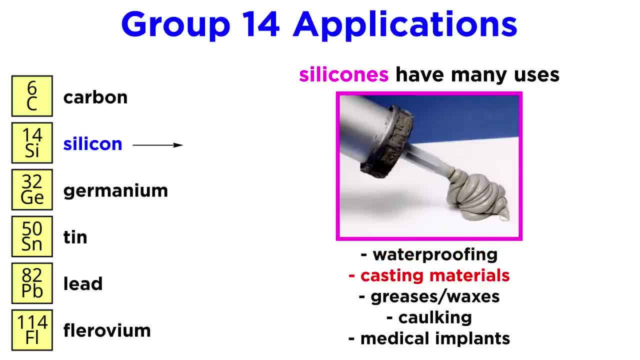 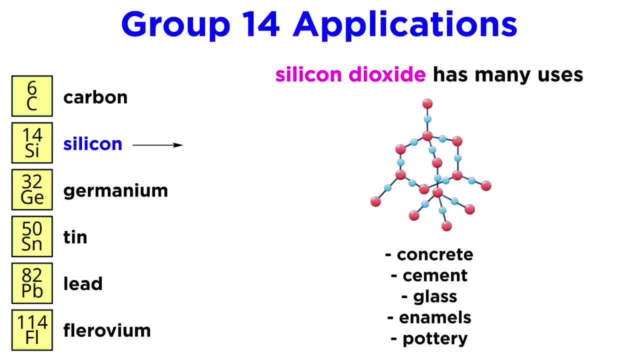 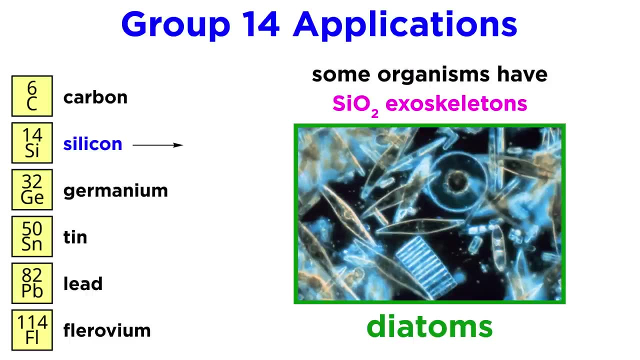 Silicones are used for waterproofing, casting materials, high temperature greases and waxes, caulking and medical implants. Silicon dioxide is used for concrete, cement, glass, enamels and pottery. Some organisms, like diatoms, even have silicon dioxide exoskeletons. 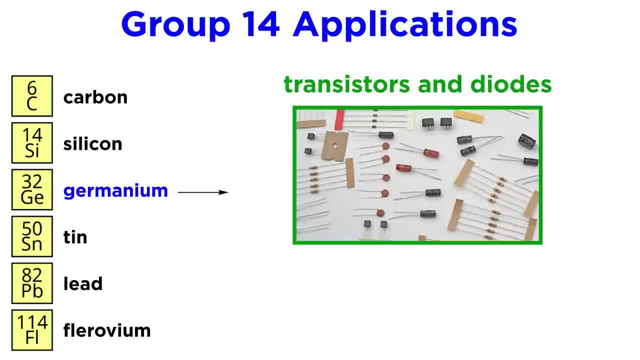 Germanium first found application in transistors and diodes. Germanium oxide has a high index of refraction and low dispersion, so it is essential in keeping light within fiber optics. For this reason it has replaced titanium oxide in glass for fiber optics. 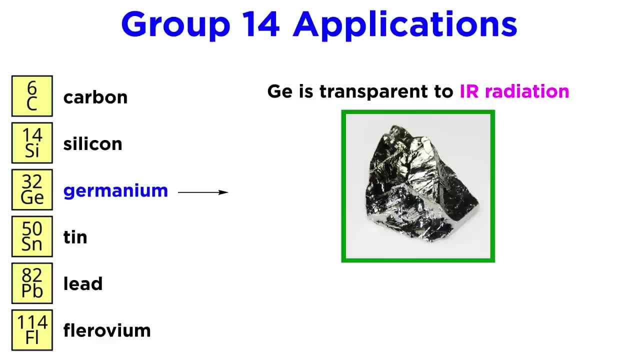 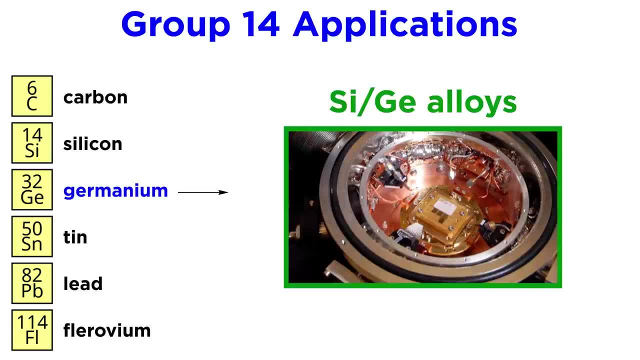 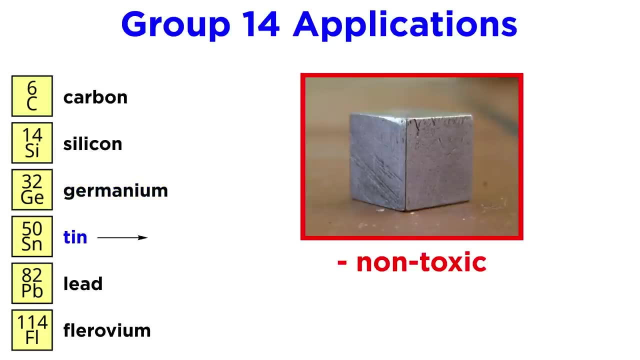 Germanium is also transparent to infrared electromagnetic radiation, so it is used for IR optics, thermal imaging cameras and night vision equipment. Silicon-germanium alloys are also finding use in microchips. Tin is an interesting metal as it is non-toxic, does not rust and is very easy to melt and 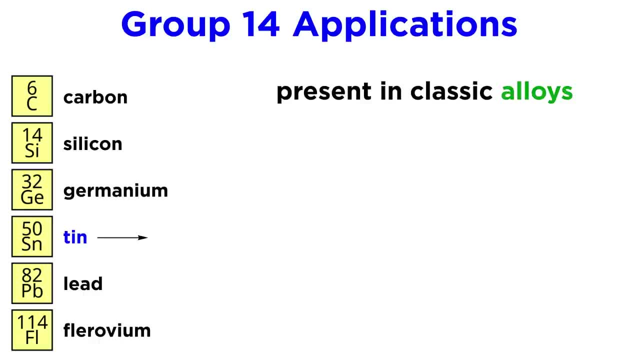 cast Tin is present in some of the most classic alloys, such as bronze, an alloy of tin and copper. solder, an alloy of tin and lead, and pewter, an alloy of predominantly tin and mixtures of other metals like silver, copper, zinc and manganese. 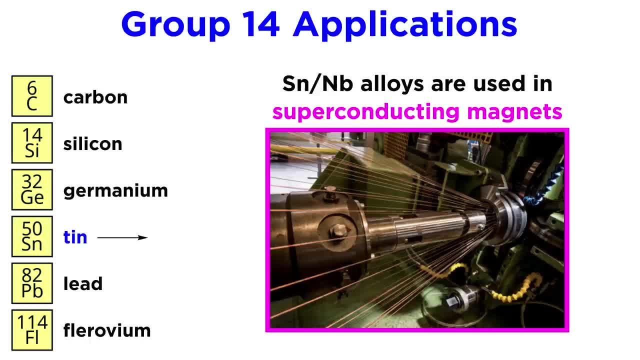 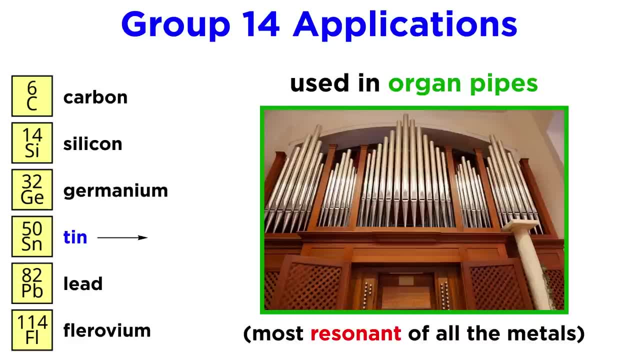 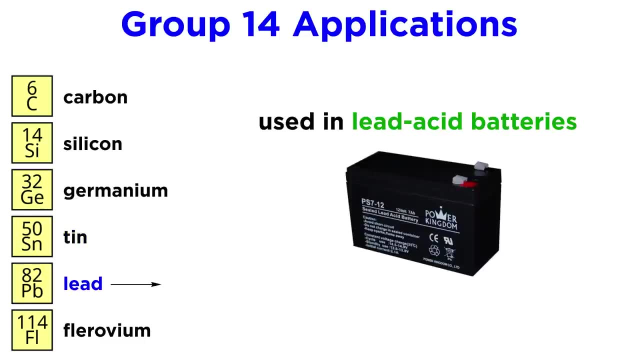 Tin- niobium alloys are used in superconducting magnets. Tin plating of iron, lead, zinc or steel helps prevent corrosion, And tin is used in organ pipes. as it is the most resonant of all the metals, Lead has tremendous application in lead-acid batteries. 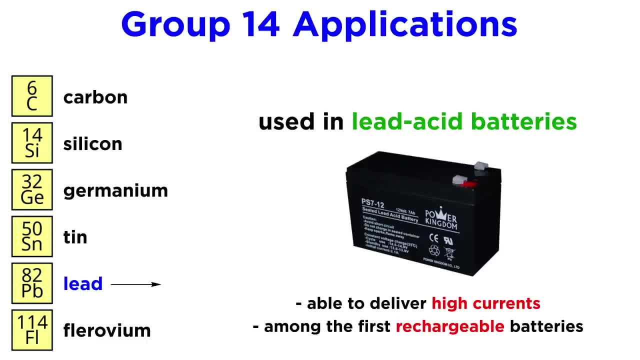 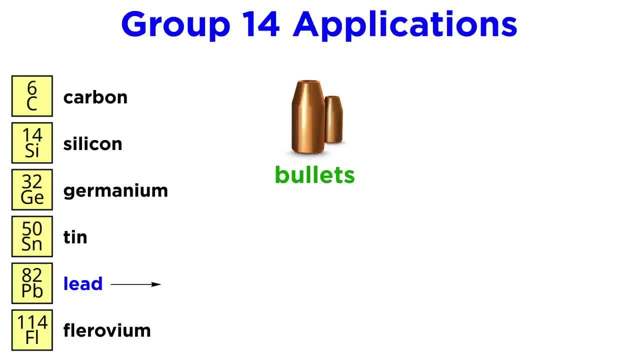 These are capable of delivering high currents and were among the first rechargeable batteries. Lead is used in bullets due to its high density, while being soft enough to not jam the barrel. Lead is also used in pewters, in radiation shields and was long used for pipes as these. 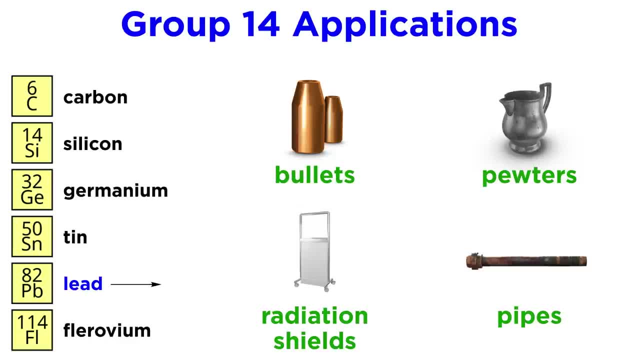 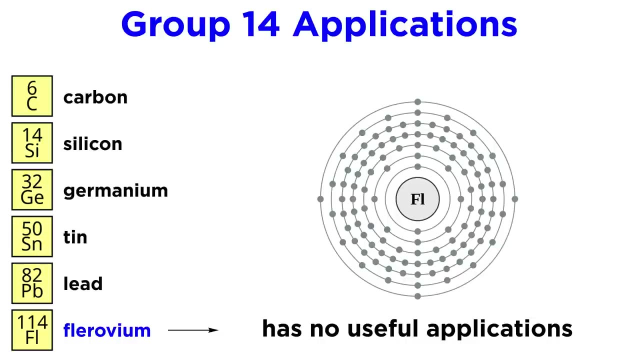 are easy to weld and repair and they do not corrode very easily, though some corrosion does occur, which is why lead pipes are no longer advisable for carrying drinking water due to the potential danger of lead poisoning. And, as we mentioned, fluorovium has no useful applications due to its extremely short half-life. 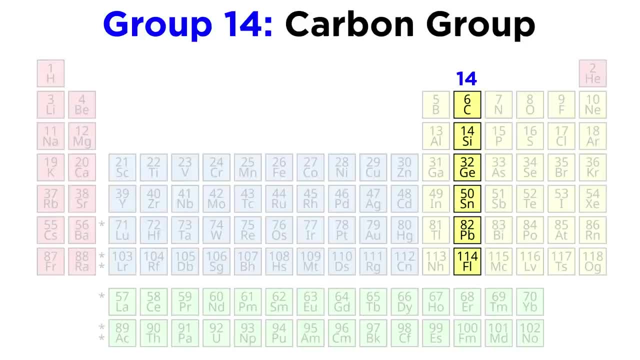 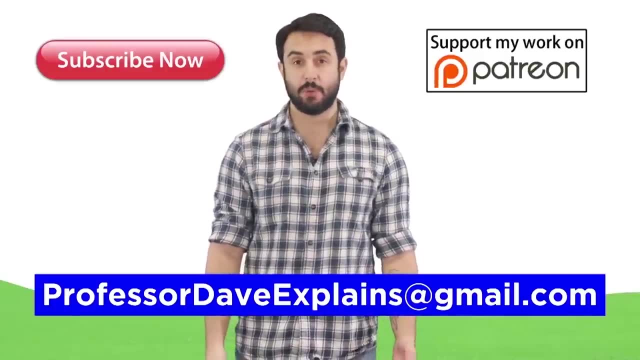 And with that we wrap up another group from the periodic table. Thank you for watching and, as always, feel free to email me professordaveexplains at gmail dot com. 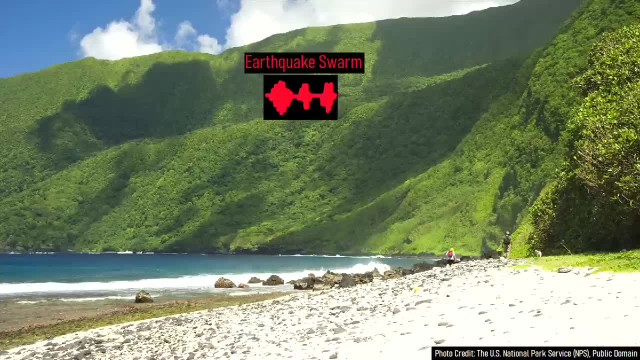 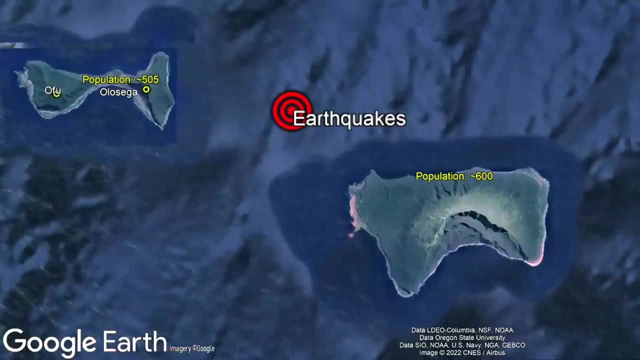 Beginning on July 26th of 2022,, a swarm of earthquakes began shaking three islands within American Samoa. Over the next several weeks, an increasing number of quakes were widely felt on the island of Ofu, Olu-Sega and Ta'u Due to a lack of thorough seismic. 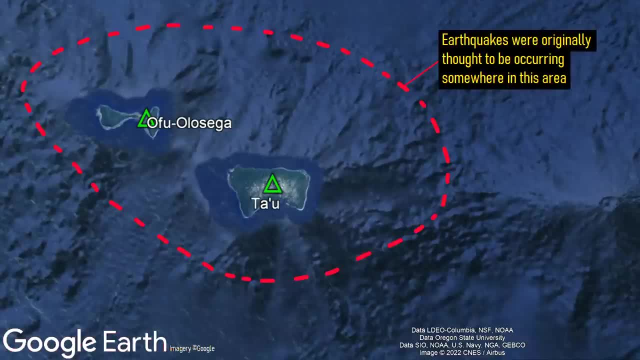 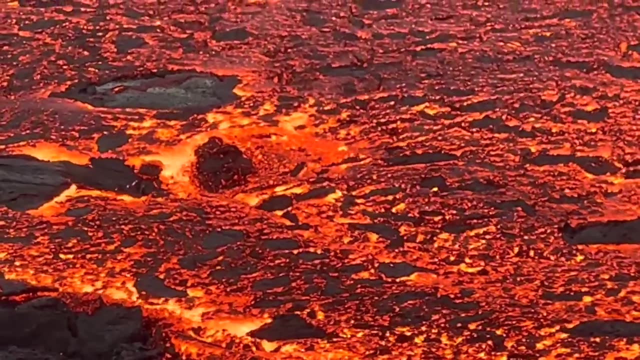 equipment in the area, it was initially difficult to locate where the earthquakes were originating. Regardless, it was almost a certainty that the up to 30 quakes an hour which were occurring, the largest of which were in the upper magnitude 3 range, were magmatic in origin. 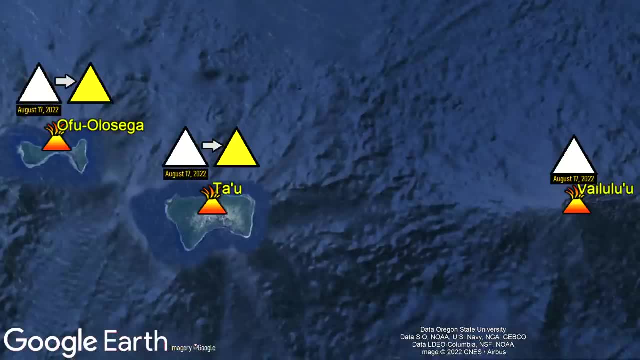 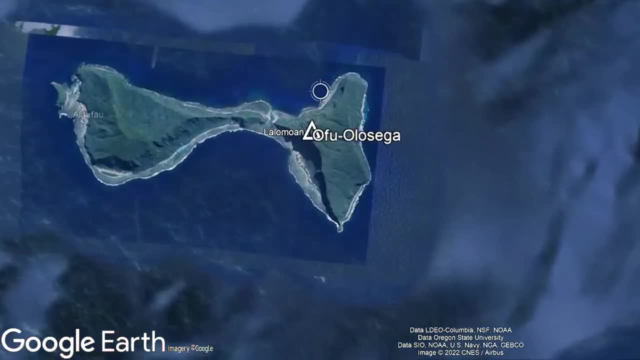 As a result, the alert level of both the Ofu Olu-Sega and Ta'u volcanoes were raised from white to yellow on August 19th. Seven days later, the color code at Ofu Olu-Sega was downgraded back to white as the quakes were determined to not be originating from.